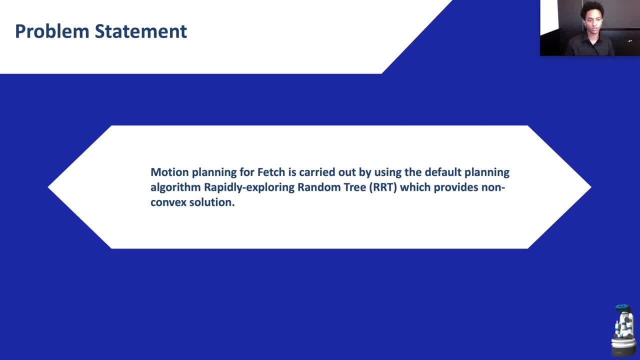 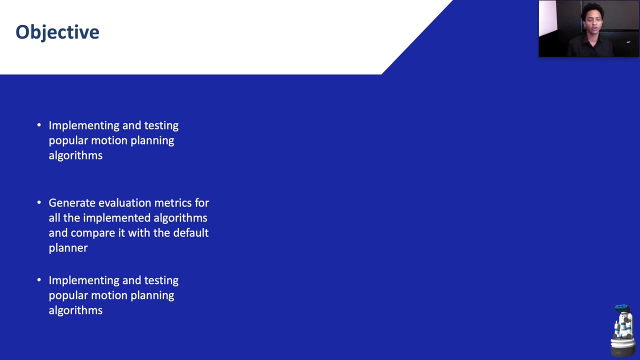 RRT gives a non-convex solution, meaning the solution found or the generated trajectory might be different even though no changes have happened in the environment nor the task. The objective of this project is to implement alternative planning algorithms. The results generated in this project include the following. 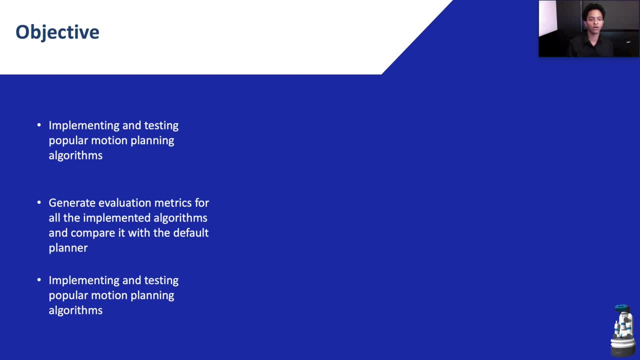 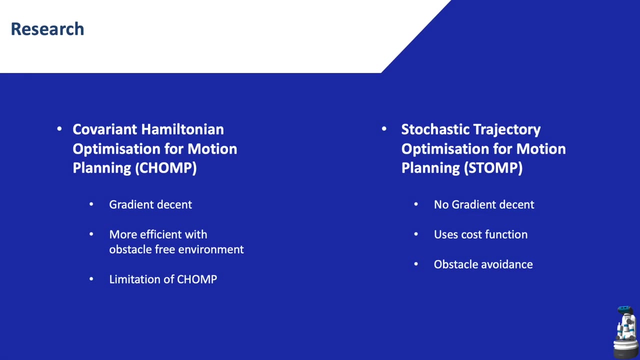 The results generated from the experiments will then be used to design evaluation matrices for these implemented algorithms, which then will be compared to the default planner RRT. This project also gives roboticists and research students the opportunity to work with more planners. Most of the research was done in part A of this project to explore the planning algorithm alternative that can be implemented in the Fitch robot. 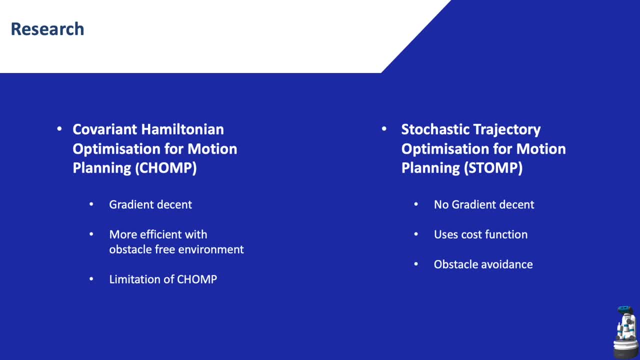 The results will be distributed in the following 2 algorithms. The first one is the Covariant-Homogeneous Optimization for Motion Planning, or CHAMP, which is a planning optimization algorithm that is able to generate a trajectory in multidimensional space using a functional gradient technique known as the gradient descent. 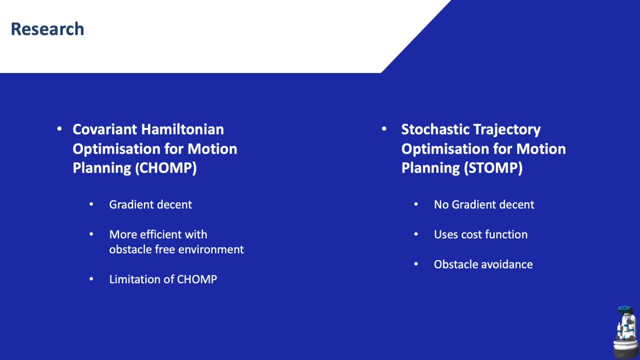 It operates more efficiently in environments with no obstacle. I don't have a term for gradient descent. Let me tell you more about this program. gradient descent is that it causes jump planner to be stuck in a local minima if obstacles were added to the environment. the second planner is known as stomp short for stochastic trajectory. 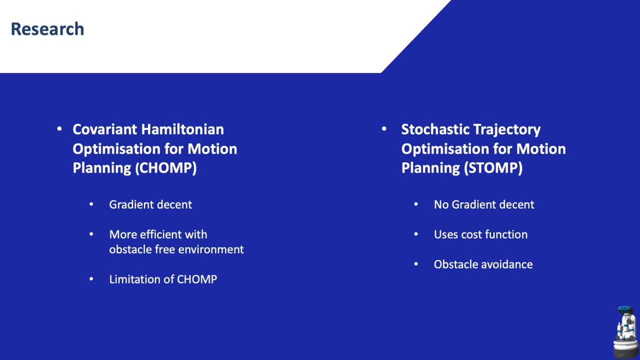 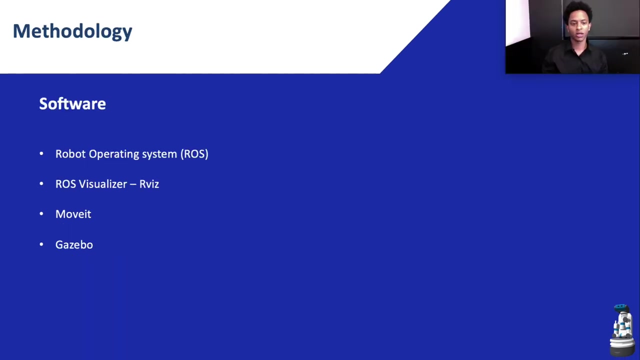 optimization for motion planning. unlike trump, it does not require gradient descent, which solve the problem of stacking in a local minima. instead, stone use a cost function to satisfy object avoidance and motion smoothness. this project is mainly based on software and the software used, our robot operating system, also known as ross harvest, which is a ross visualization tool. 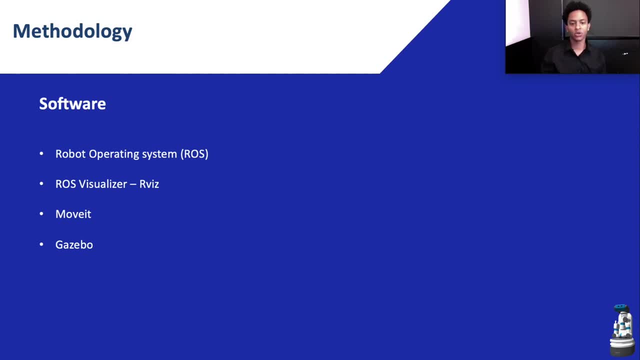 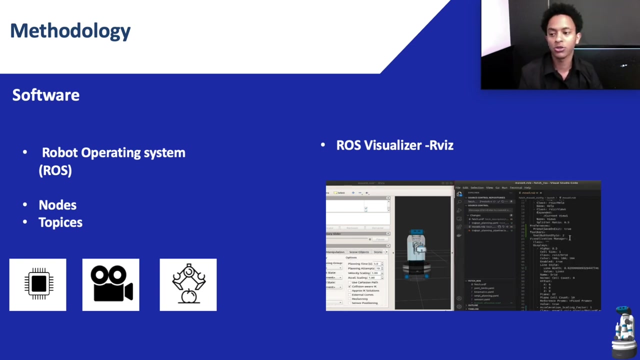 move it framework for motion planning and the simulation was done by the gazebo simulator. now let's take a brief look at the functionality of this software in this project. robot operating system, or ross, is an open source software. it uses topics and nodes to communicate the three parts of any robots which 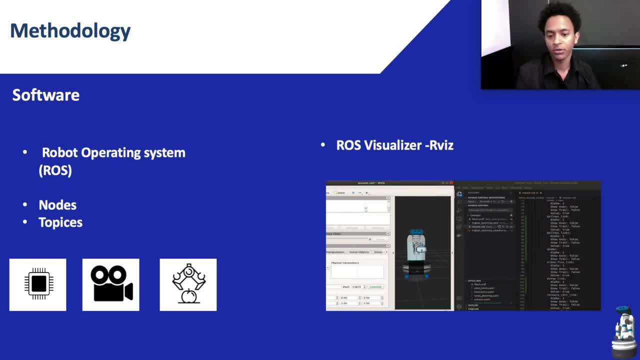 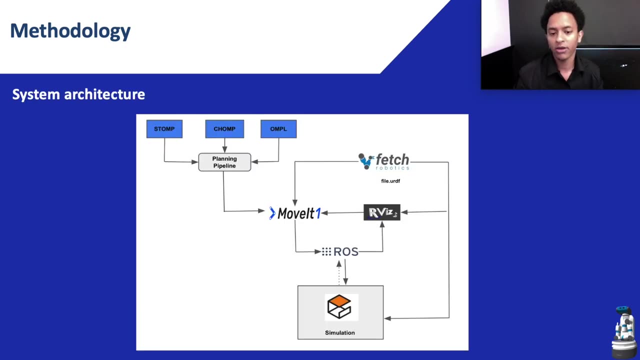 are the actuator, sensor and the controller. ross visualizer, or harvest, is a powerful ross tool that helps us to visualize the planning scene as well as makes the debugging process much easier. the following diagram is a high level representation of the whole system that shows how all software used are communicating. 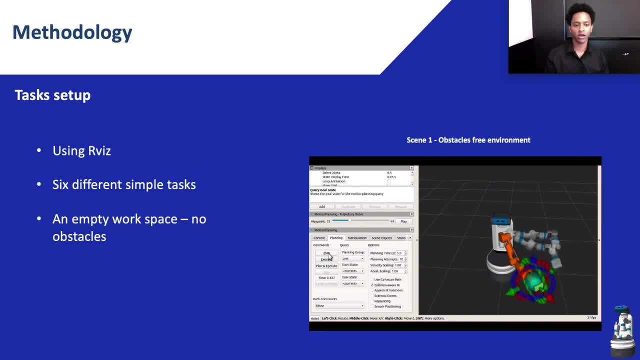 using harvest. six different tasks were designed to carry out the testing for the three planners rrt, trump and stomp. the complexity of the task increases when we add obstacles into the planning scene. as you can see on the screen in scene 1, the planning for this task is simply done in obstacle. 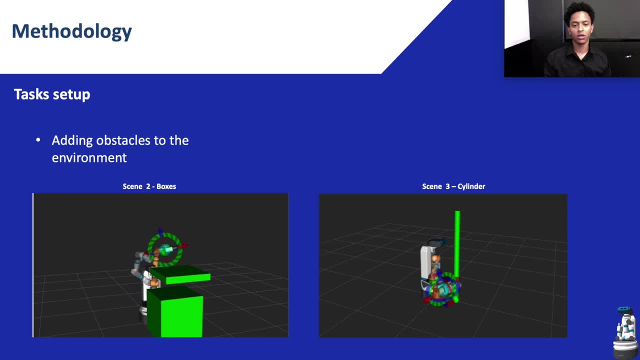 free environment. the difficulty is then increased by adding boxes to the workspace, as shown in scene 2, which is considered easier than scene 3, where the object is located very close from the robot manipulator. it is important to remind you at this point that we have only changed the environment or 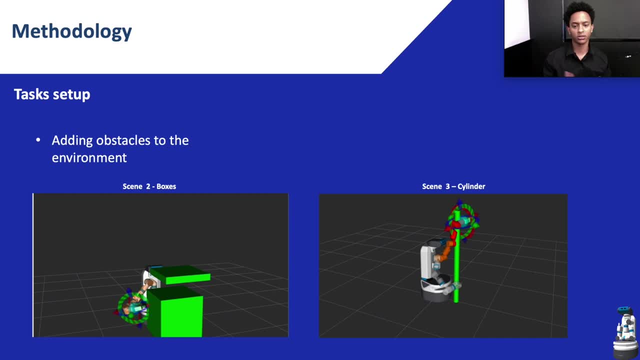 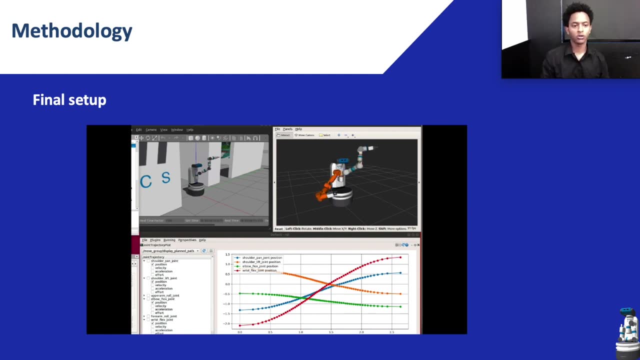 the planning scene and all six tasks are still the same. here we can see the full setup for the planning scene. the video shows. harvest tool on the right of the screen is connected to the simulation of the fish robot in gazebo. on the left we can see that the user is carrying out some motion planning. 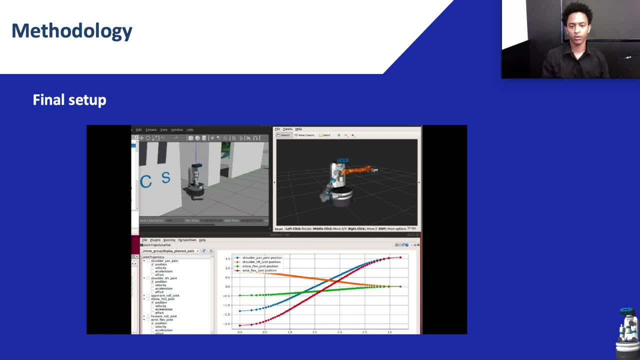 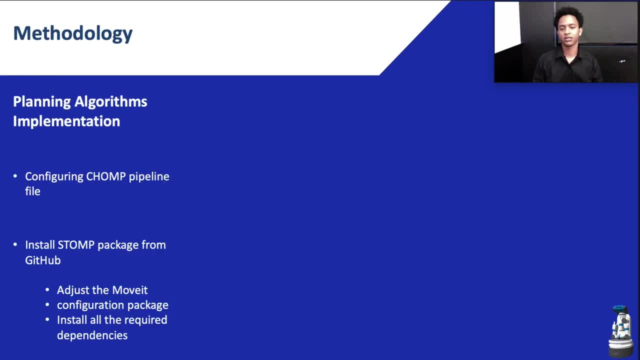 which is then being executed on gazebo. at the bottom of the screen we can also see the plan trajectories for the specified joints. let's take a step back, because we cannot plan for these tasks without using planning algorithms. hence trump and stump were implemented in the move it framework. to plan for these design scenarios for chum, the required pipeline file. 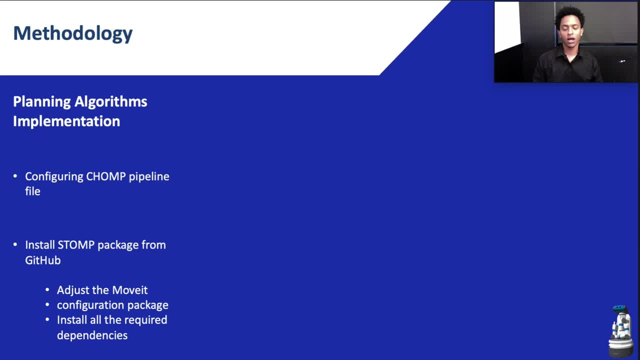 was set up for the planner to operate or move it. however, for his thumb the planner needed to, or the package of the planner was installed from github and the required files adjusted so that it can work with the movie group, and all the required dependencies were also uninstalled. after we explain: 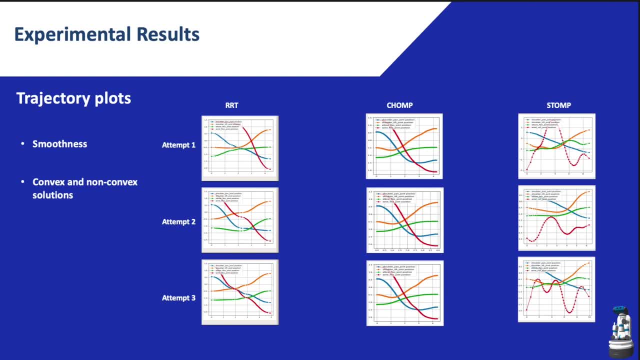 what's required to plan the work, and the options are the following: the main structure is that you can choose to plan for natural or not, depending on the type of project or the type of design. the plan is usually based on the plan he has prepared for the project. you have to do a sort of 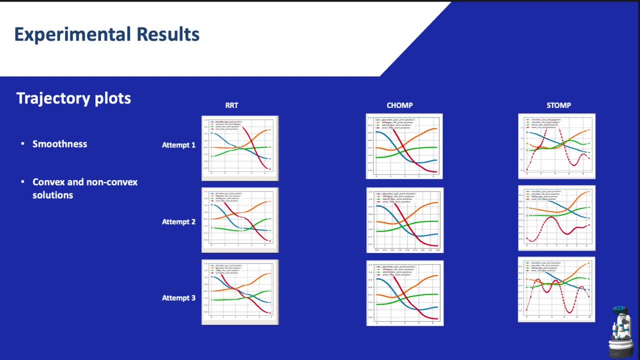 analysis and evaluate the plan as much as possible. the results can be submitted by using the pattern of data and the, but that's the point of the plan. the plan is based on the model and it's the best to have a plan in place to manage the data. that's also a very good way to manage the quality of the. 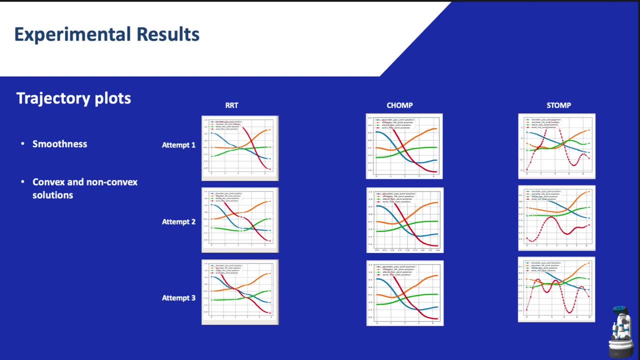 convexity. As I mentioned earlier, RRT planner is a non-convex because it generates different trajectory for the same task. Let's start with the trajectory quality By carrying out a number of attempts of the same task using each of the three planning algorithms. as it shows in the graphs, Trump is consistent. 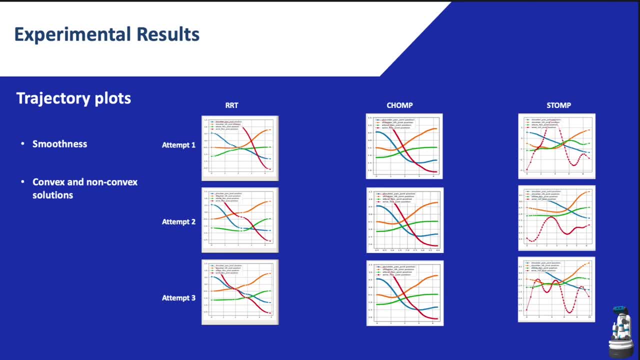 in generating the same trajectory in all three trials. On the other hand, RRT and Stomp give a different solution in each attempt. When it comes to smoothness, we can easily observe the plots, which shows that Trump is the one that generates the smoothest trajectory, followed by RRT and the last one is Stomp. 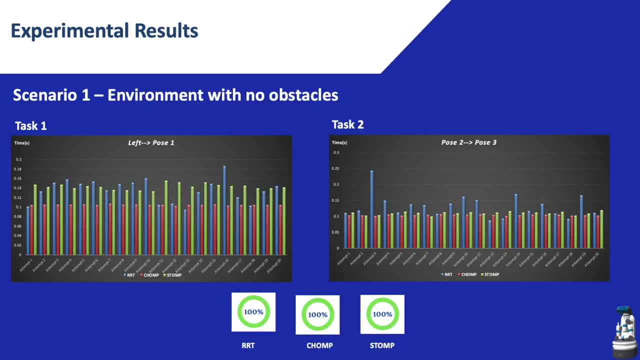 Next is the planning time and the success rate which we were taking in the three different scenarios. The bar chart illustrates the planning time for each of the planning algorithms tested in the obstacle-free environment, completing 20 attempts for both task 1 and task 2.. 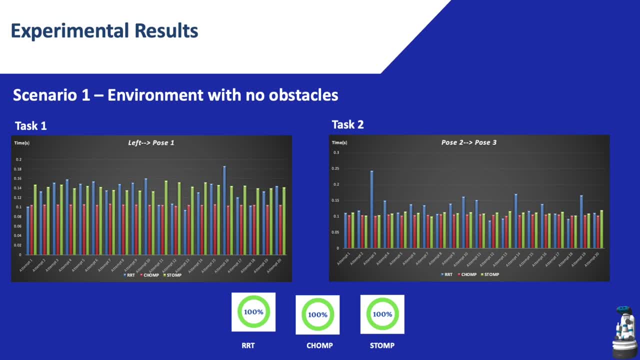 With no obstacles. Trump planner has the least time taken to plan for all 20 attempts, While RRT has the longest time to complete or to compute the trajectory for both tasks. Also, all planners completed task 1 and task 2 with a 100% success rate. 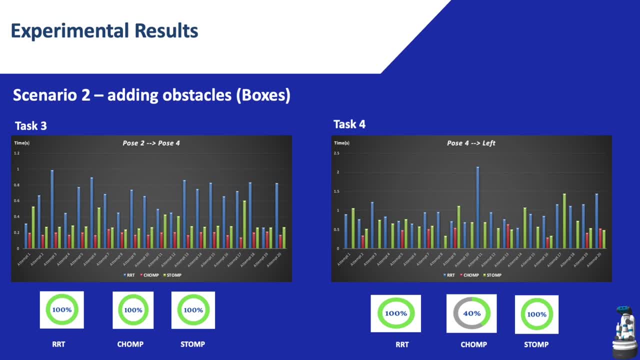 Next, we added some obstacles to the planning scene. As we can see in task 3,, there is a significant difference between, or in the planning time for RRT and the other two tasks. In task 3, the planning algorithm is Trump and Stomp, with Trump still having the least.